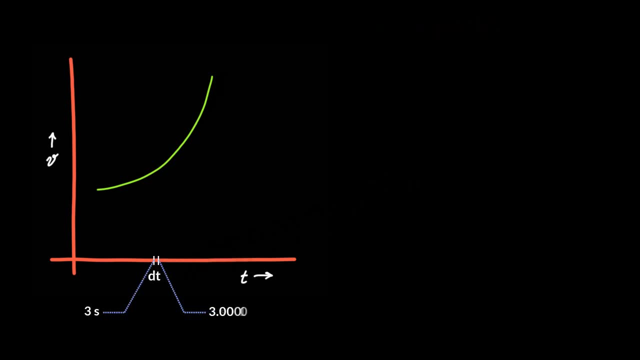 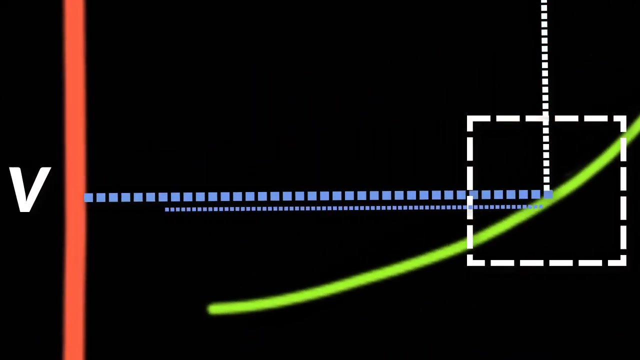 say between 3 seconds and 3.00001 seconds. and let us say, in this time interval the velocity of the particle is v. Well, you could say that within the time interval dt also, the velocity is changing, and if you zoom in you can see that it indeed does change, But the change is so small. 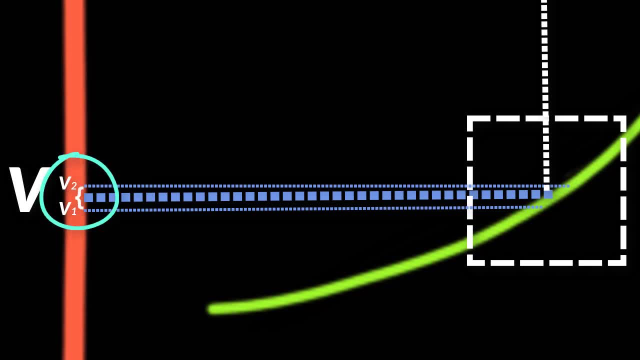 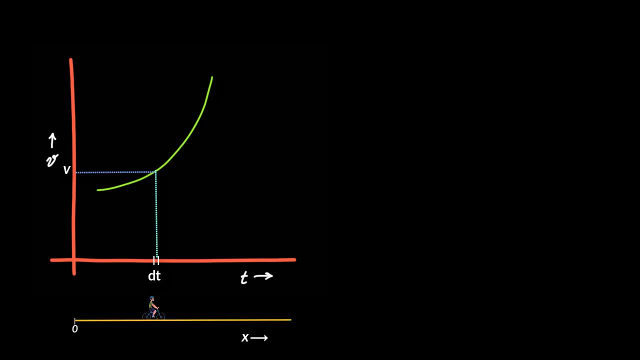 that we can agree to assume that it is one single value, v, and so the displacement in time dt, can be given by the usual equation, that is, displacement is equal to velocity into time. or here, displacement dx is equal to velocity into time, So displacement is equal to velocity into time. 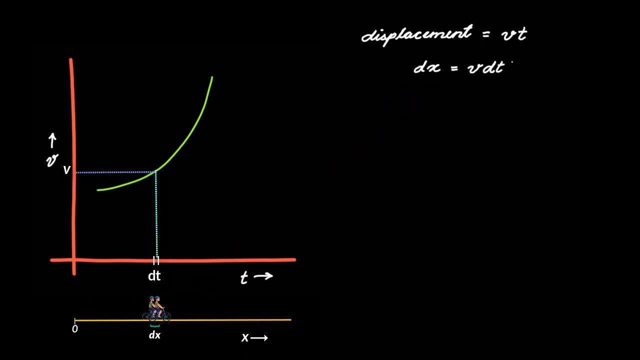 But then you will observe that v times dt is nothing but the area of this rectangle that has width, dt and height v. So we can say that in a velocity time graph the area of a rectangle with width, dt and height v gives the displacement of a particle in time dt. 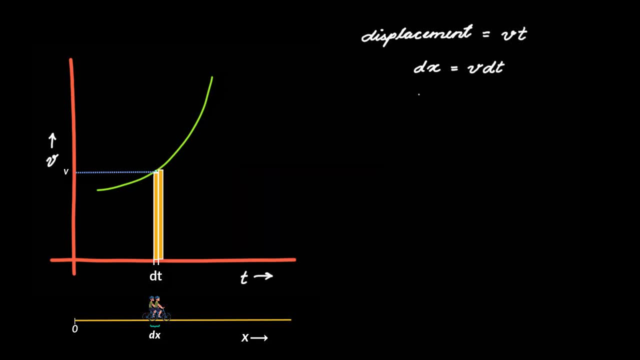 Well, we can take another time interval dt adjacent to this one, and let us say the velocity here was v dash. Then again we can find the displacement in this time as dx dash is equal to v dash times dt, and once again we see that this is nothing but the area of this rectangle. 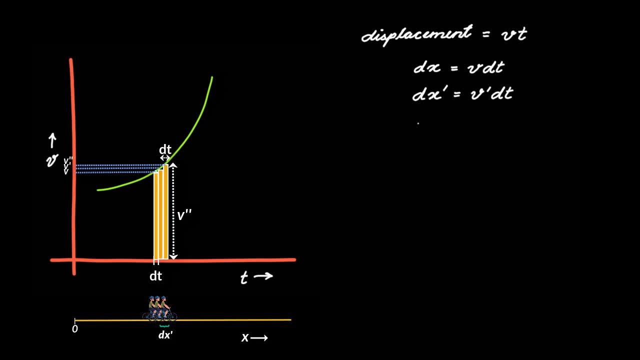 And then why not take another time period dt adjacent to this one, and say the velocity is v double dash here, Then the displacement in this time period is dx double dash, which is equal to v dash dt, which again is the area of this rectangle. So this means that if we can add up the area of 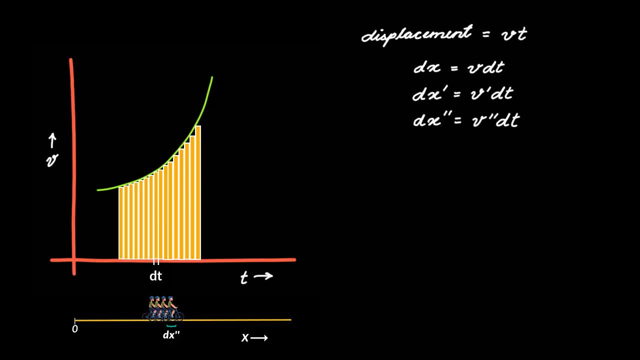 all such rectangles under this velocity time graph between time t0 and t1, then that should give the displacement between time t0 and t1.. But the summation of these several narrow rectangles would be very difficult if we try to do it ourselves. However, this can be done quite easily using a mathematical tool. 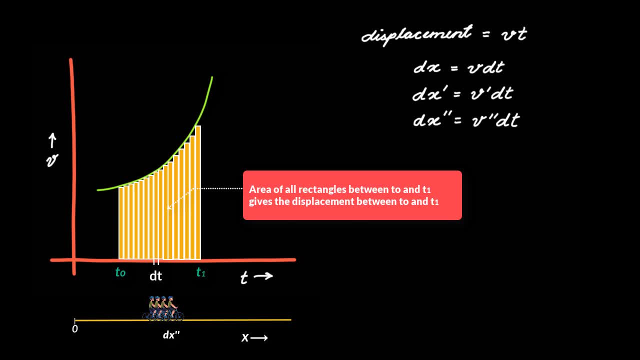 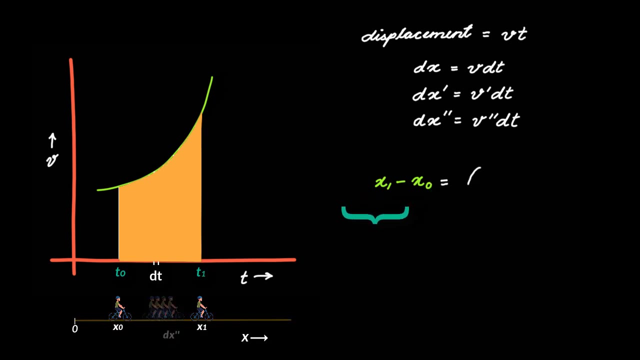 called graphical integration, and using this tool we can say that the area under the curve between t0 and t1, which is the displacement in this time interval, is given, as x1 minus x0 is equal to integral of v dt as the limits change from t0 to t1.. And here v is velocity. 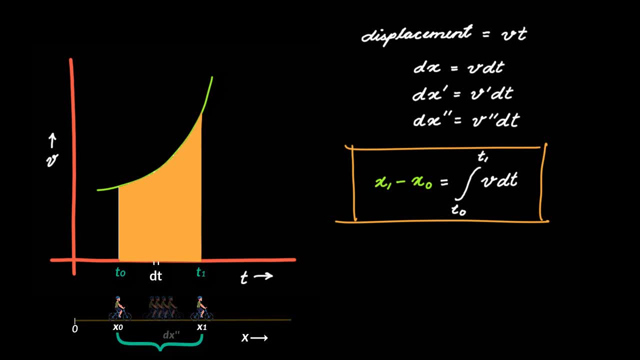 at any time, t between t0 and t1 and of course x1 and x0 are the respective positions. So this expression, you see, is nothing but the value of the area under this curve between t0 and t1.. And if we speak a little more mathematically, the right side of the equation is called a definite. 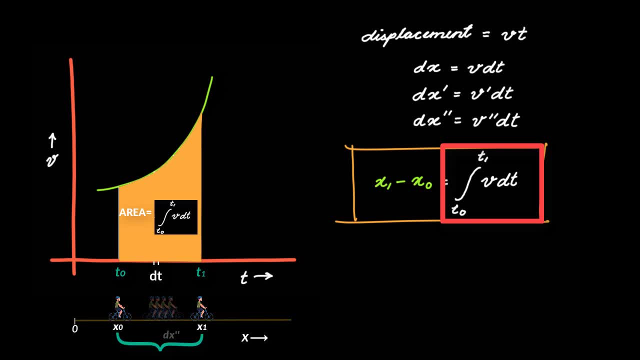 integral, which in simple words means that it gives a numerical result. So at first it might sound a little confusing, but we will get to that in a few minutes. So let us start with the integral. So what this equation is saying is: and please, 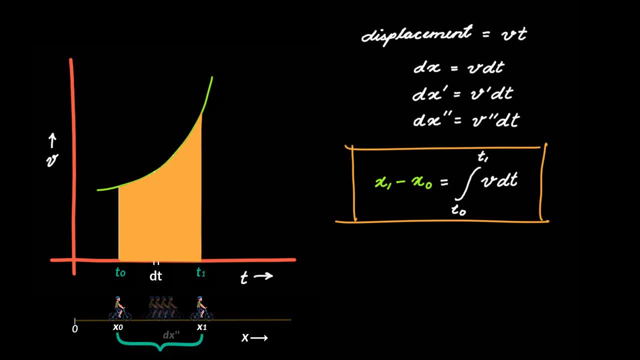 hear it carefully- that if you can find right hand side of the equation, then this value you find is a value of this area, that is, the displacement of the object between time t0 and t1.. So let us work around a simple problem that would make. 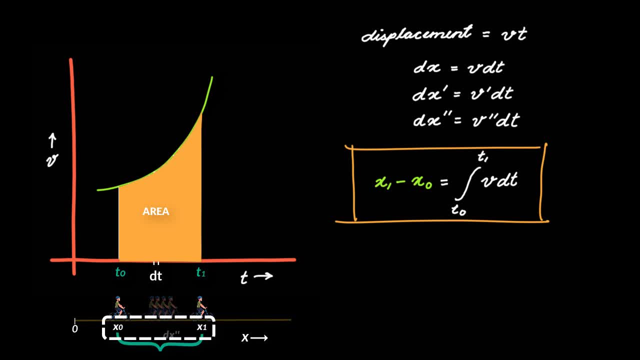 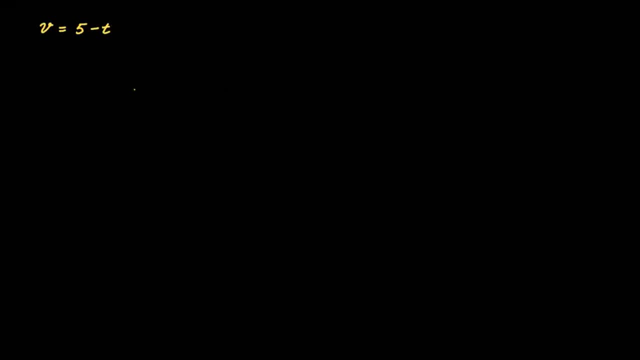 things a lot clearer for you, and the problem is that an object whose velocity is related to time, v is equal to 5 minus t, so at t equal to 0, velocity is 5 meters per second, and at t equal to 5 seconds its velocity becomes 0. and now you're asked: what is? 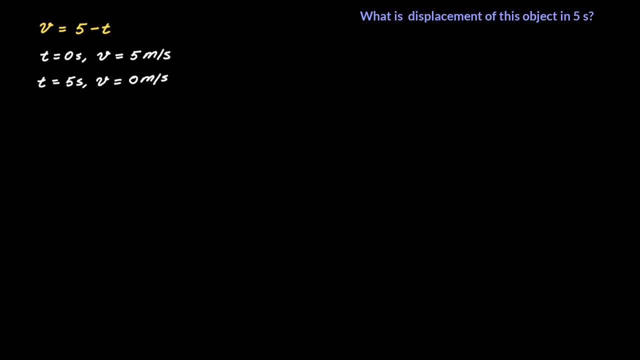 displacement of this object in 5 seconds. so let us use this graphical integration technique to find the displacement between. t is equal to 0 seconds and 5 seconds, and the first step would be to make the velocity time graph for this equation and this curve. you see, it turns out to be a straight line. so the 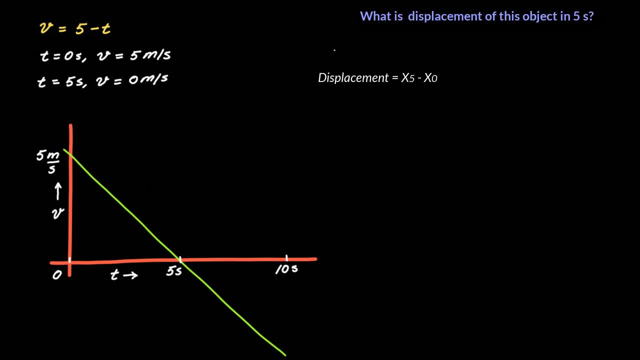 displacement can be written as x5 minus x naught, where x5 is the position at time t equal to 5 seconds and x naught is the position at time t equal to 0 seconds. then, using this formula, we do integration between t equal to 0 and 5. 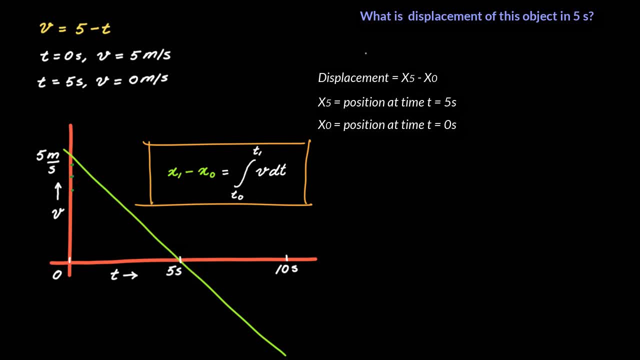 seconds, which, as we learned, should be the area under this curve or this straight line. so let us go ahead and integrate this and what we get is x5 minus x naught, that is, the displacement is equal to integral of V? DT, as the limit changes from t naught to t5, which equals integral 5 minus t DT, which equals 5t. 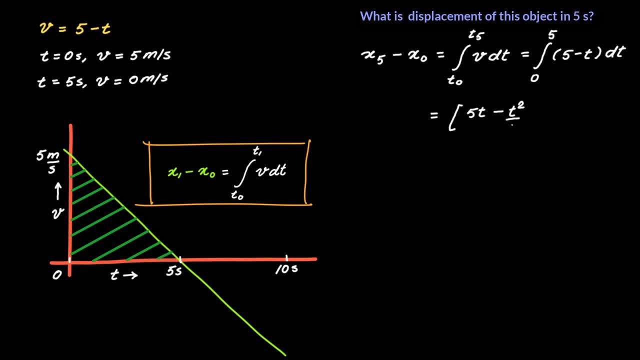 minus t, square upon 2, with limits changing from 0 to 0. so this is the total distance traveled between 0 and 5 seconds, and this then, if you calculate, equals 12.5 meters, and if you actually find the area under this straight line, 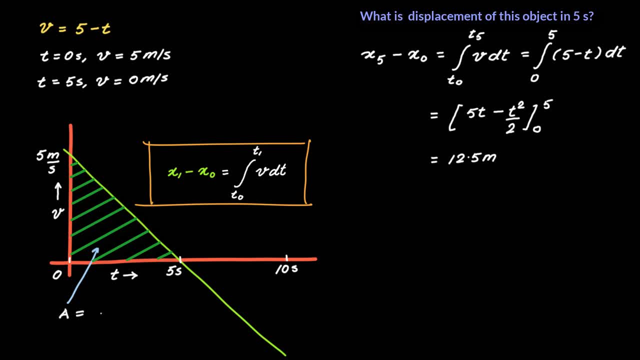 between 0 and 5 seconds. that would be half into base, into height, which is equal to half, into five, into five, that equals twelve point five units. and you find that the area indeed is the changing position or displacement between 0 and 5 seconds. now, if you are asked what is the displacement between 0 seconds and 10 seconds, that is from. 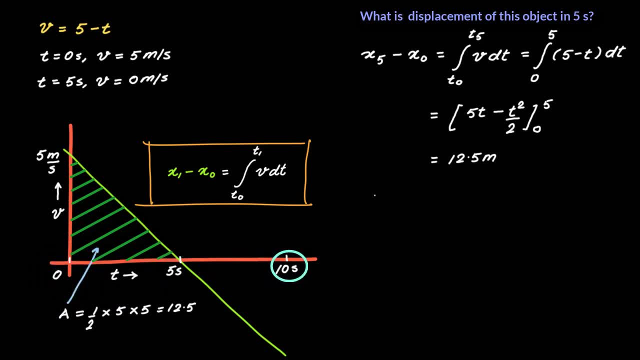 here to here. we can use the same equation but just change the limits. so what we get is x 10 minus x. naught is equal to integral of 5 minus t. dt limits changing from 0 to 10 seconds. and when you solve this, what you get is 0 meters. and the answer should not surprise you, because you see, 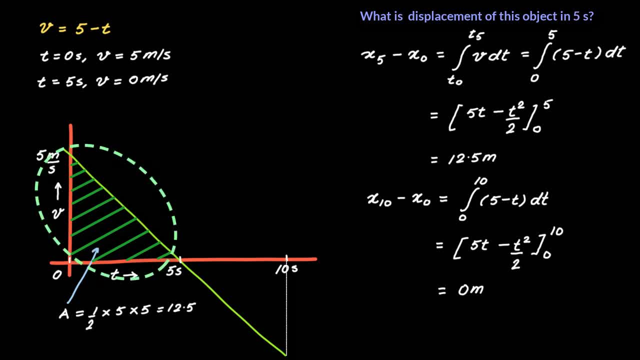 this area is 12.5 meters square, but this area is minus 12.5 meters square, so any area which falls below the x-axis would need to be taken as a negative area and therefore the two areas add up to give you zero area and therefore zero displacement. and if you were to interpret 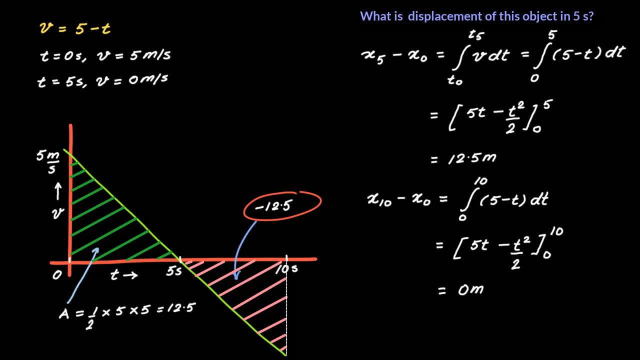 this result? it basically means that the particle moved in one direction, from position x naught to x5, between 0 and 5 seconds, and if you were to interpret this result, it basically means that seconds. but then between five seconds and 10 seconds it came back to its initial position. 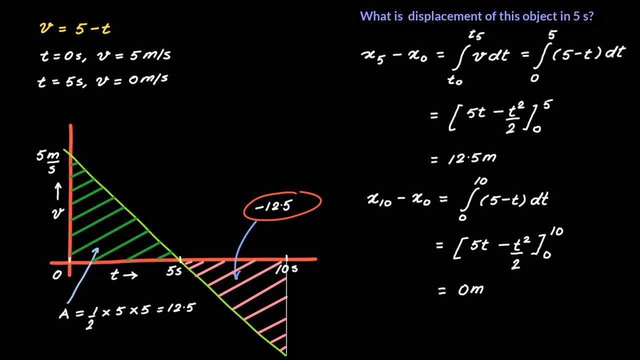 that is x naught, thus making the total displacement zero. So if you are given a velocity time graph like this and you are asked to find the displacement between t equal to zero and t equal to 20 seconds, you will find this area, this area and this area and then add them up. 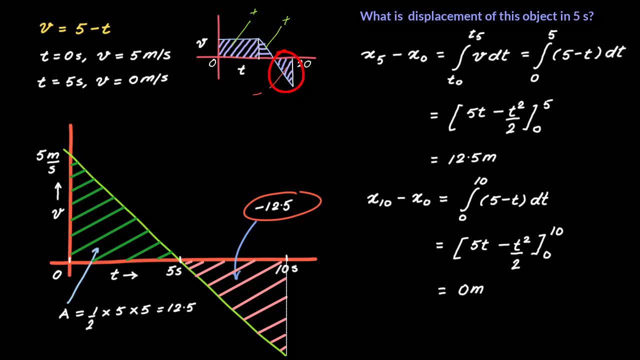 But you'll just need to remember that this area needs to be taken as a negative number because it is below the x-axis. Now you might say that why do we need to do this integration when you can just find the area of this triangle using simple geometry? Well, you would be. 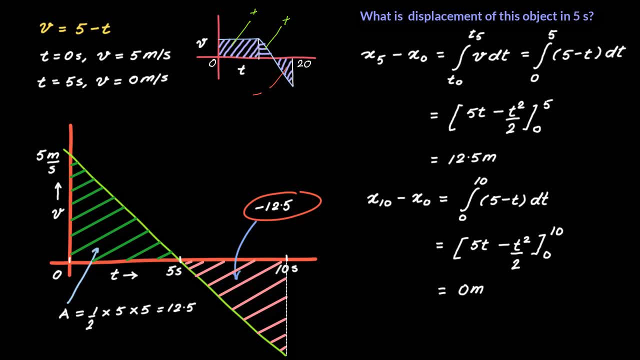 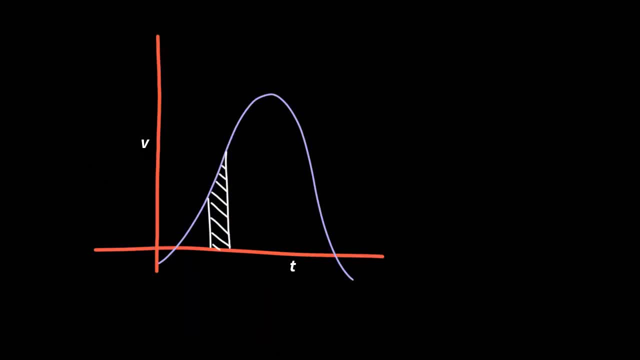 absolutely right And probably that's a way you should solve a problem like this. But if you are given a velocity time graph which looks like this- that is, the relationship between velocity and time is not linear- And say it is, v is equal to 2t squared, or v is equal to, say, 3e to the power 1.5, then it is. 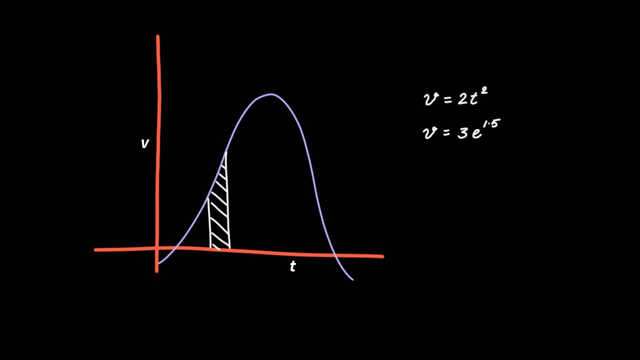 not possible to use simple geometry to find the area under the curve, And you will have to use integral calculus to find the area. So for this part of the lesson, whatever we have learned so far, I would like you to remember one thing very clearly, And this might sound repetitive, but 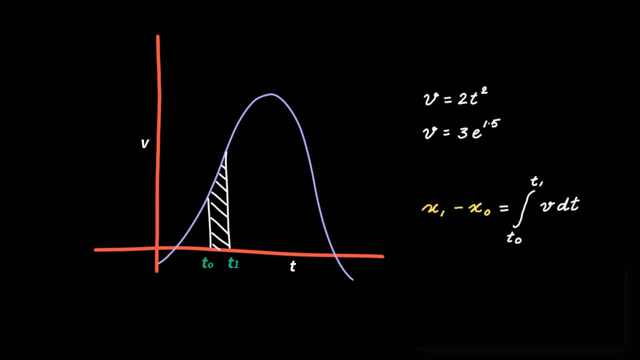 very important. That is, the area under the curve between two times represents the change in position and not position itself, at any time. And if you want to find the position at the end of the time interval, that is, at t1,, all you need to do is use the same. 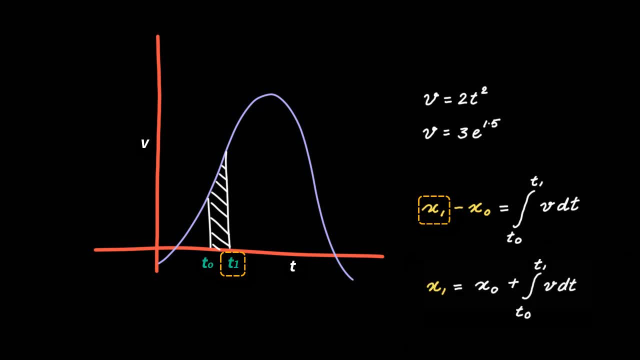 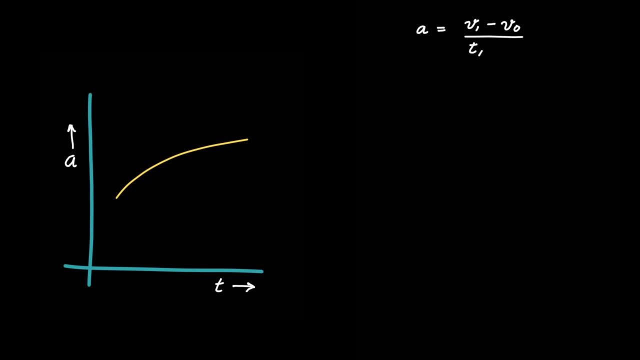 equation, but take x0 to the right hand side. Okay, let us now move on to the next topic, And that is: what does the area under an acceleration time graph give? So let us start with a familiar equation: a is equal to v1 minus v0 upon t1 minus t0, or v1 minus v0 is equal to a times t1 minus. 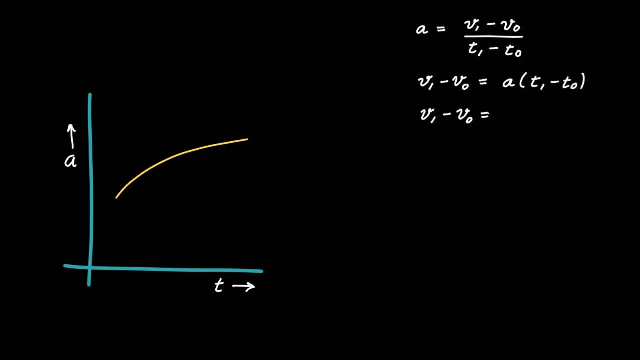 t0, or simply a delta t. So this expression is the change in velocity between t0 and t1, because you can see on the left hand side it is a difference between the two velocities. Now, if you see an acceleration time graph and take a very small time interval- dt and multiply,